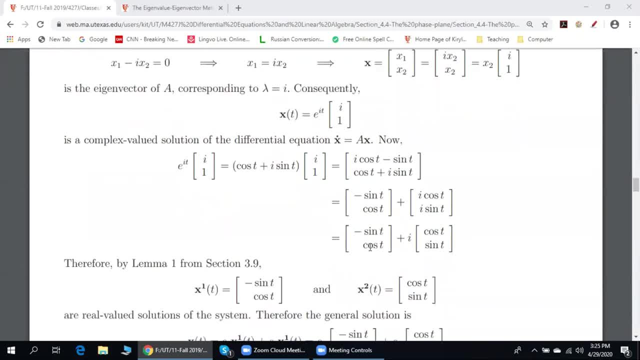 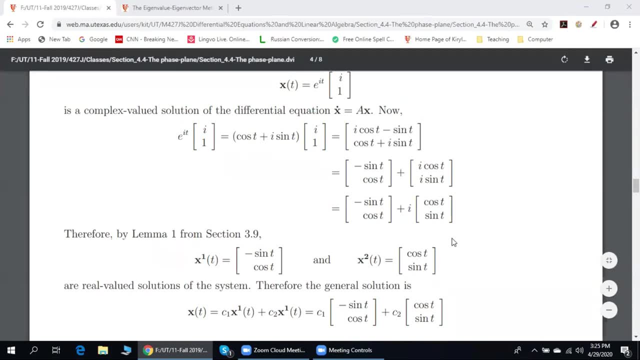 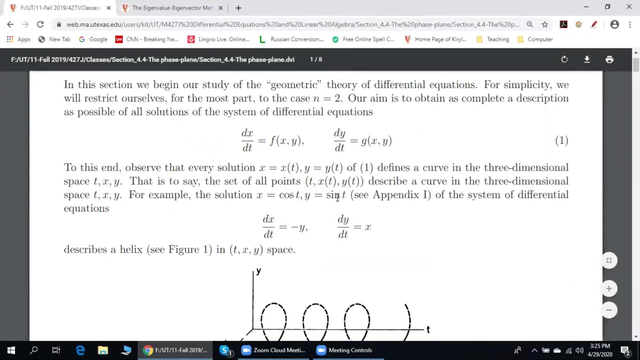 order to rewrite this as the sum of two pieces. This is particular solution number one. This is particular solution number two. So particular solution number two is cosine t sine. t Means x of t is cosine, y of t is sine. It's exactly what we have here: X is cosine, y is sine. Now, in order to graph this solution: 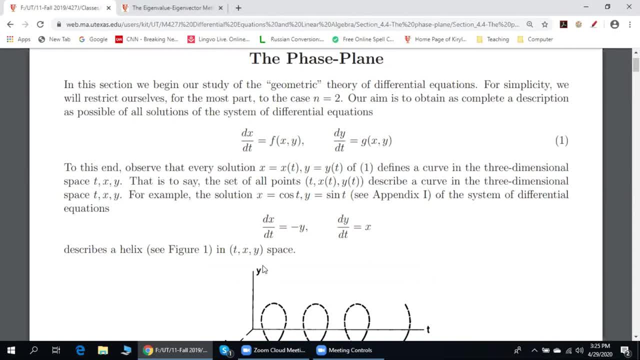 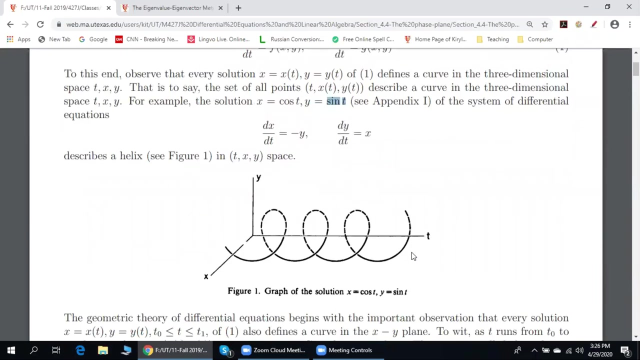 let us consider the following. The following: triple T, x, y. So if we replace x by cosine and y by sine, we'll get the following: triple T- cosine of t, sine of t. I claim that this set of all such points trace a helix in. 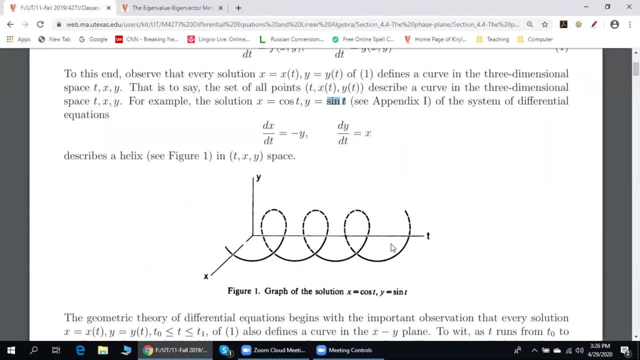 three dimensions And this is what we need If we convert this each other in one dimensional space. this is y. Note that for any fixed value of t, since x is cosine and y is sine, and because cosine squared plus sine squared is one, 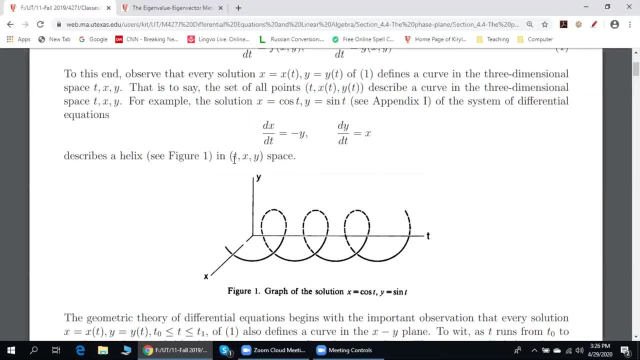 for each fixed value of t, the corresponding point on this curve will become sine. and because cosine squared plus sine squared is one for each fixed value of t, the corresponding point on this curve will be the following: be a point on a unit circle with a center at the origin. If we cut this curve by, 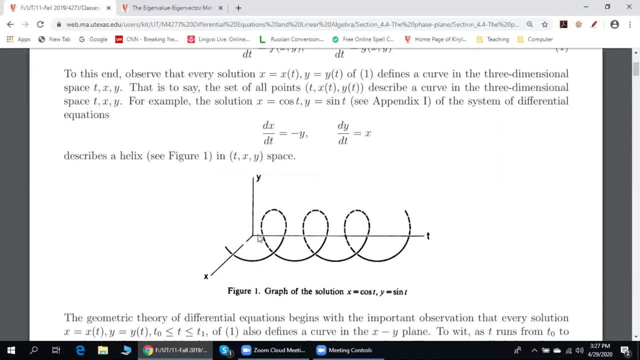 the plane which is orthogonal to the t-axis means which is parallel to the x-y plane. So once again, fix some T. See this three-dimensional curve. by a plane that goes through this point and which is parallel to the x-y plane, We'll get only one intersection point, This: 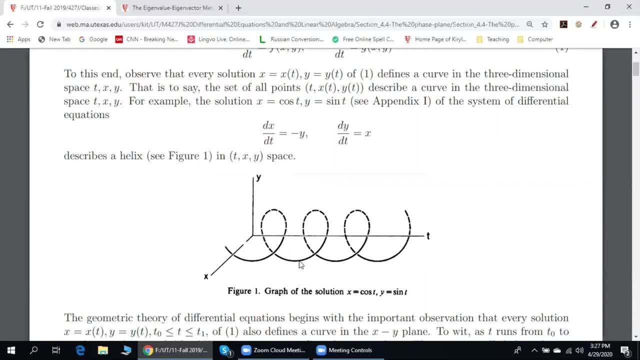 intersection point is a point on the Dunar escaped, the unit circle, with the center at the origin, because x squared plus y squared is equal to one. Now, when we change t, this point will go along the circumference of this circle. Therefore our curve is a helix. 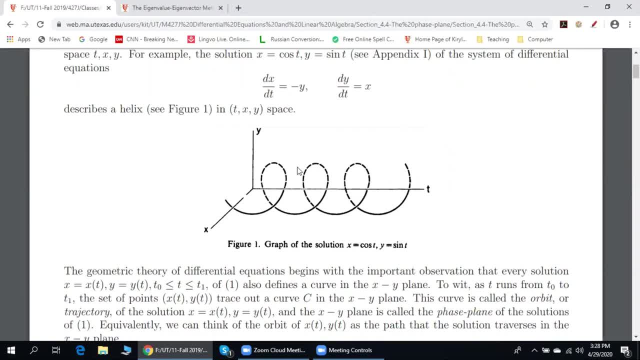 Now, for the same reason, if we consider the projection of this curve on the x-y plane, we'll get the unit circle with the center at the origin. And now terminology: We call the x-y plane face plane. We call the projection of our curve on the face. 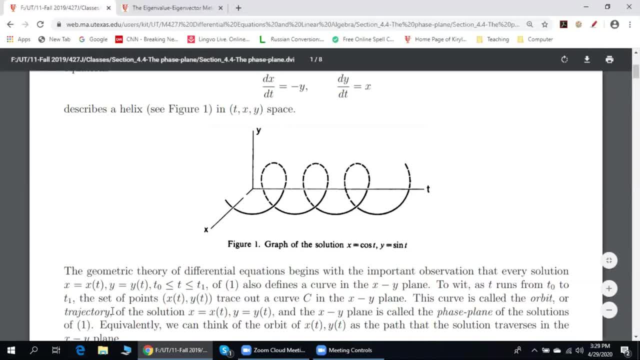 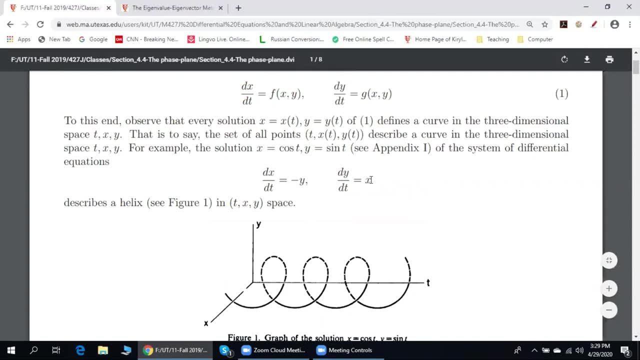 As I mentioned, we're going to explain the orbit or the trajectory. So the orbit of the solution of our system is a unit circle with the center at the origin. Any questions about example 1?? If you scroll to the appendix, Mr Kiro. 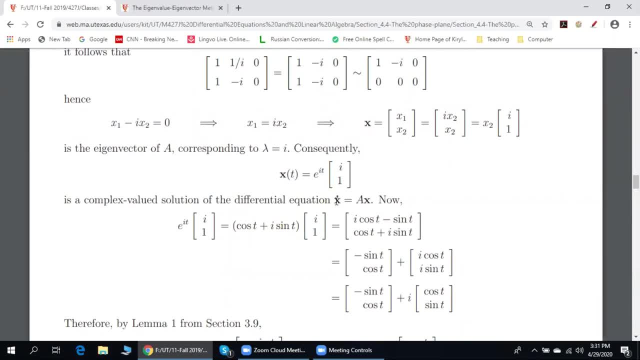 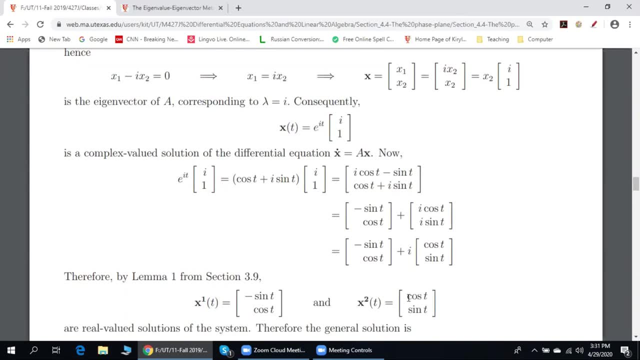 So, if you scroll down, So I understood that x is equal to x2, i and one, it's an eigenvector. and then, very shortly after, it says consequently, that it's equal to e, to the power of it, and then, in brackets, i and one. i don't where did the e to the it come? 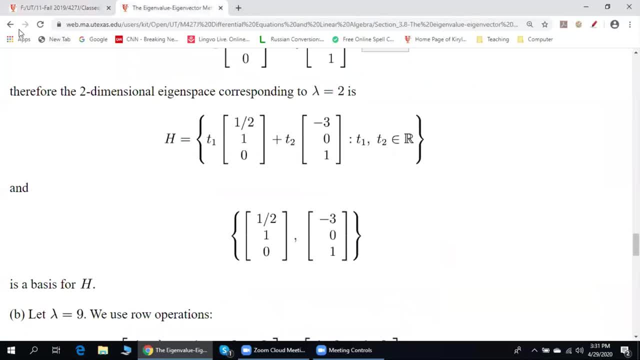 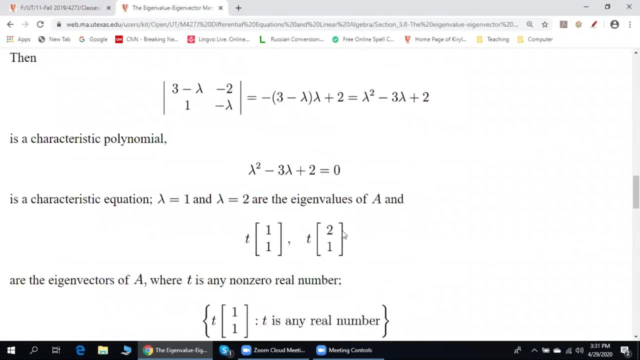 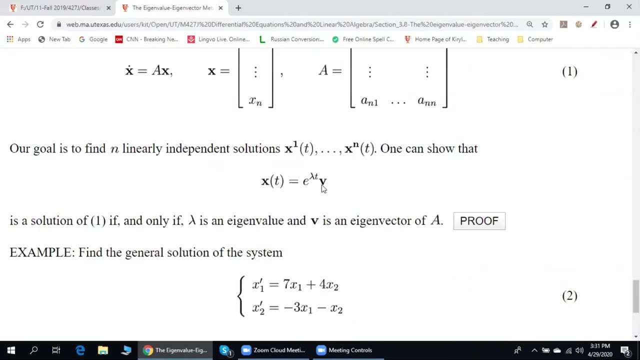 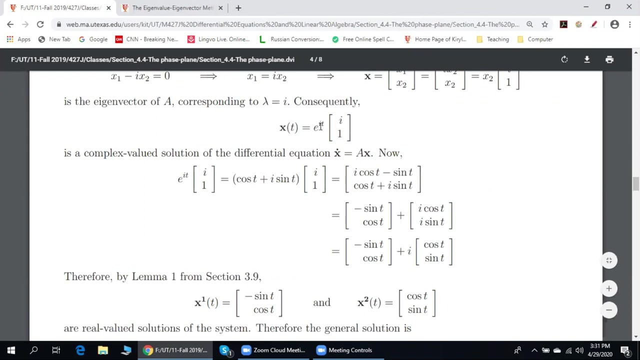 from, so we apply the standard procedure. let me go back to first section 3.8. according to section 3.8, a particular solution can be written as e to lambda t times v, in our case: a lambda is i. this is how we come up with e to it. a lambda is i, i see. okay, like this: 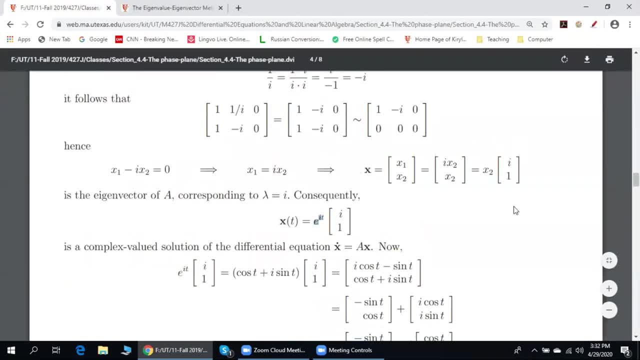 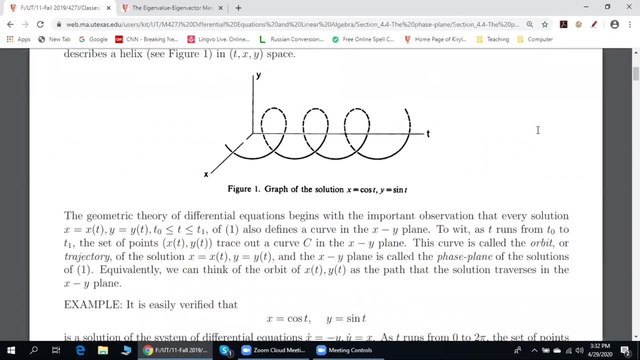 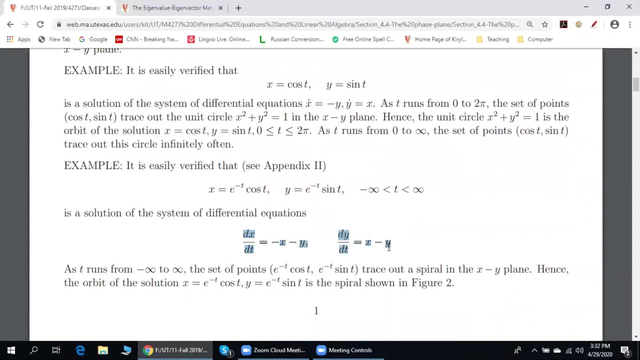 and v. is this according to what is written here? okay, okay, yeah, okay, i got. thank you. so, most important thing, the orbit is the projection of a three-dimensional curve on the xy plane that we call face plane. here's example number two. consider this system of equations. in appendix two we show: 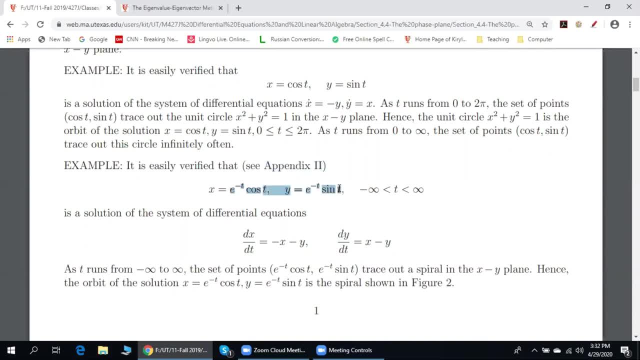 that its particular solution is this: now, if we square both sides here and square both sides here and then add the resulting equation, left hand side will be x square plus y square. right hand side will be e to negative two t, because we square and then in parenthesis, cosine square plus sine square, since cosine square plus. 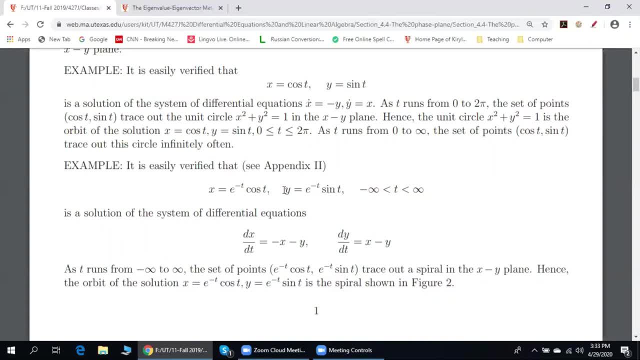 sine square is one. the right hand side becomes e to negative two t. so if we square both sides here, so we square both sides here, and add up these two equations on the left hand side we get x square and then you can make it easy to follow the tough one, because it's because z quotient in Boolean. 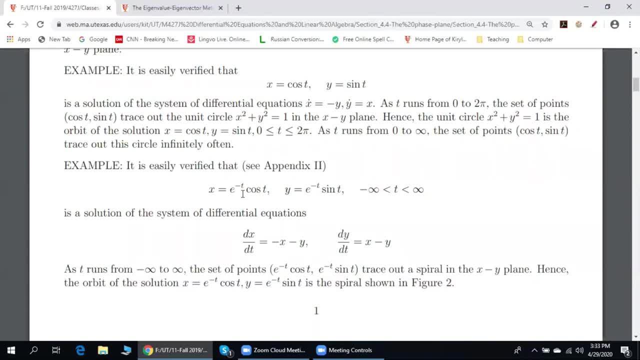 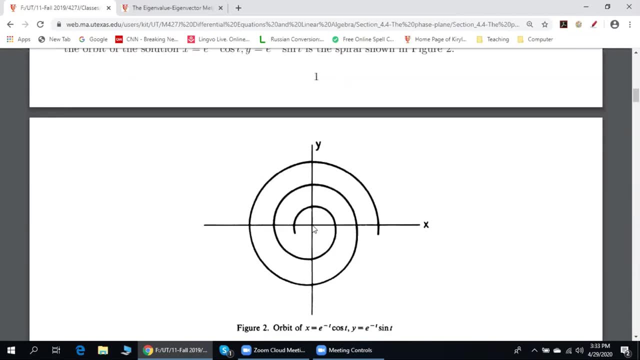 on the right hand side will be x squared up here, a percent plus plus y squared. so get x squared plus y. on the left hand side, e to negative two t. this L is a point of sure prediction because the therefore君 from the tıyla there- well, this expires- did. then you can just out of the fact that 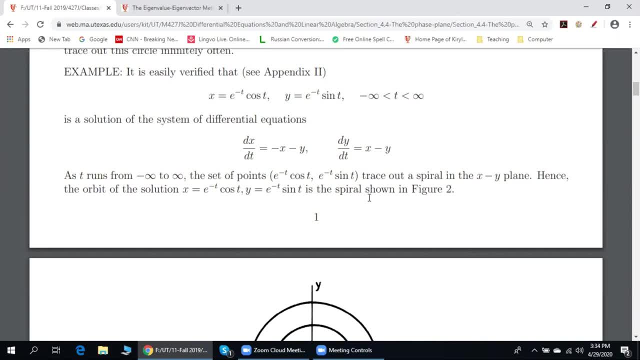 the negative, for x is nothing but a philosopher, because that's theisha that치가 is so important. well, here's another characteristic which is doing: is you multiply both sides here and add up this two equations: on the thatcha side, we get x squared plus y squared on the right. 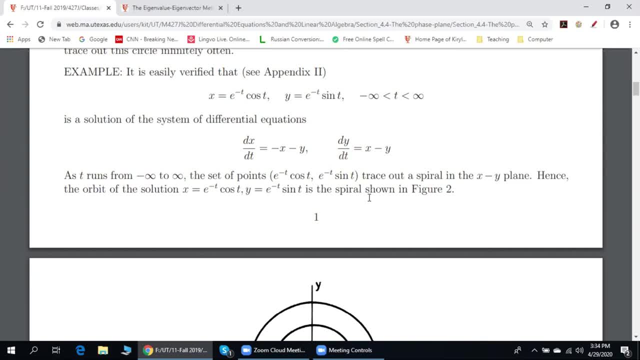 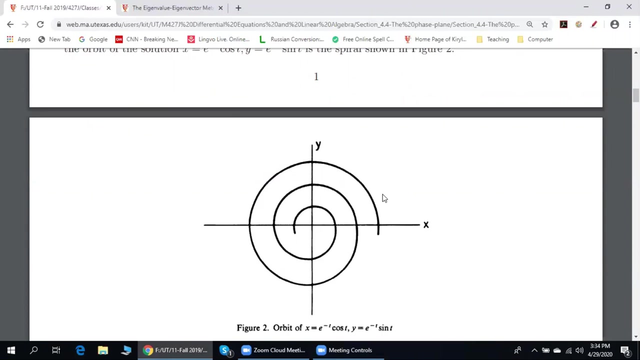 which means if t increases, if t goes to infinity, e to negative, 2t decreases and goes to zero. observe that for any fixed t, our equation is an equation of a circle of radius e to negative t. we basically consider the set of points. each of these points belongs to a circle and the radii 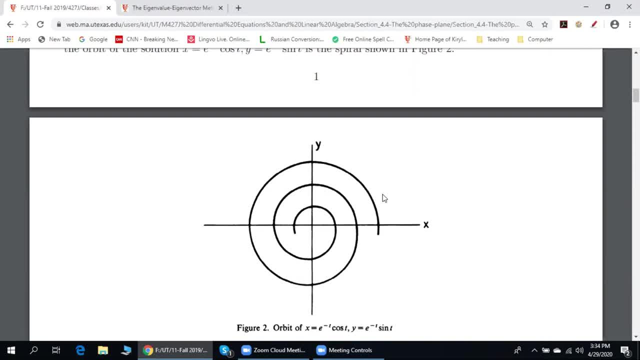 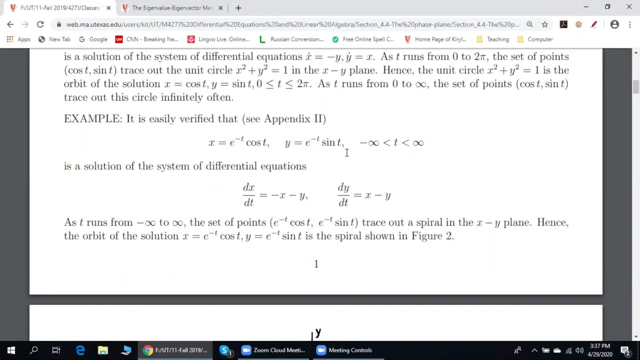 of these circles decrease and go to zero. thanks to this, we trace a spiral that converges to zero guys. any questions here? uh, can you re-explain how you know it looks like a spiral again? well, let us try it in a different way. think about this. fix some t, for example. put t is equal to zero. 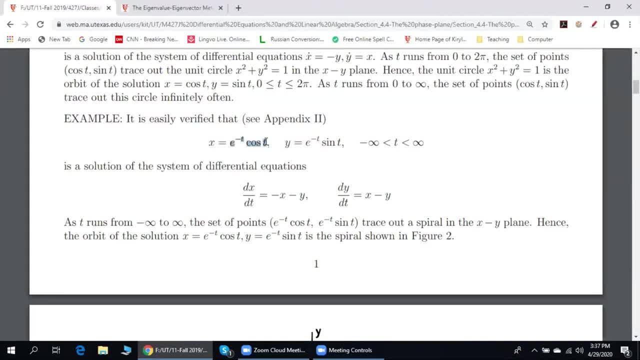 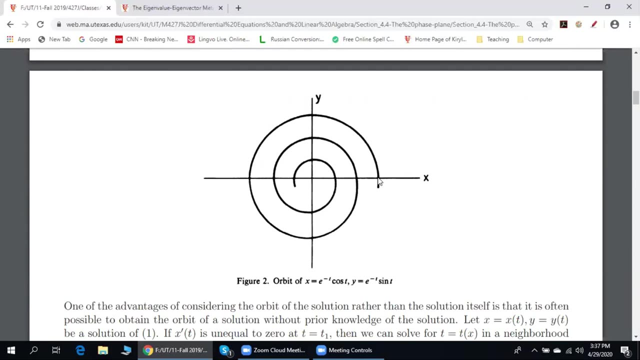 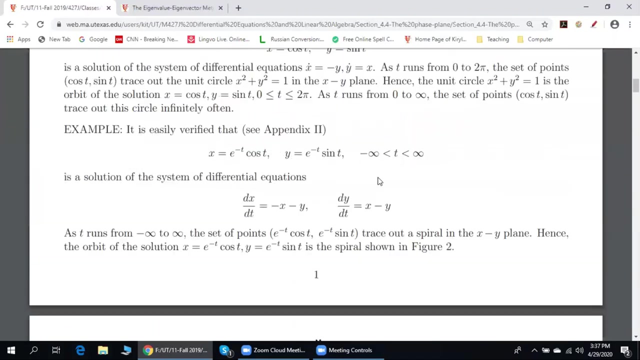 if t is equal to zero, the right hand side here will be one, the right hand side here will be zero, correct? so we'll get a point with coordinates: x is equal to 1, y is equal to 0. we will get this point correct. yes, now let us increase t. let us put, for example, t is equal to pi over two. if t is equal to, 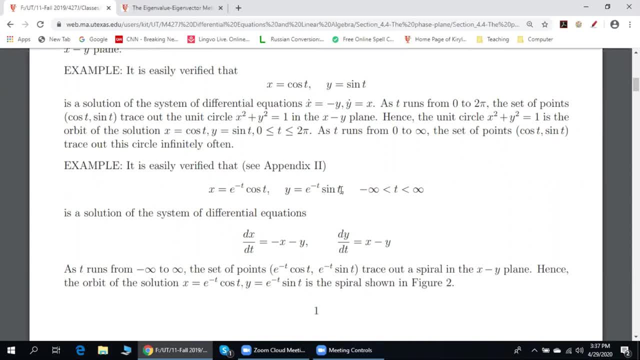 pi over two. sine of pi over 2 is 1, cosine of pi over 2 is 0. agree, yes, so if t is pi over 2x is zero, y will be e. 2 minus pi over 2 is 7 x, i will get 5. 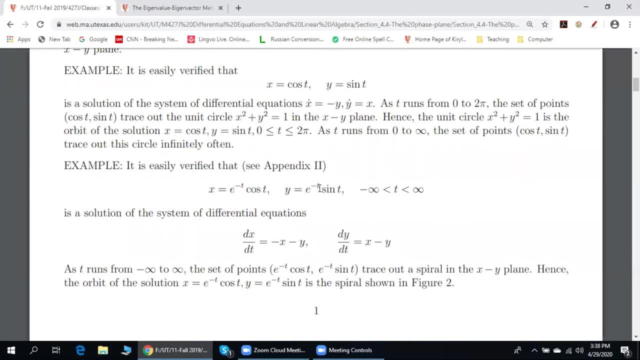 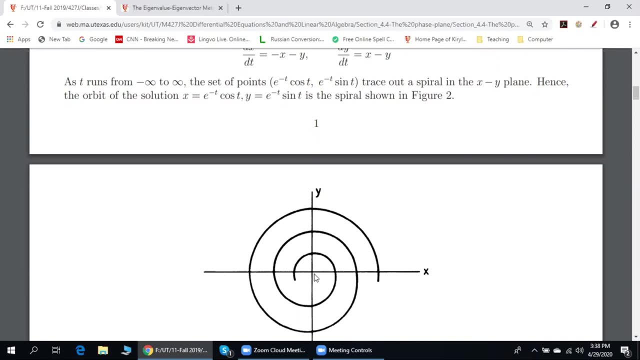 2 negative pi over 2.. Correct, Yeah, So we will get this point and observe that this distance is 1.. This distance is e to negative pi over 2, which is lesser than 1.. So this distance is lesser than. 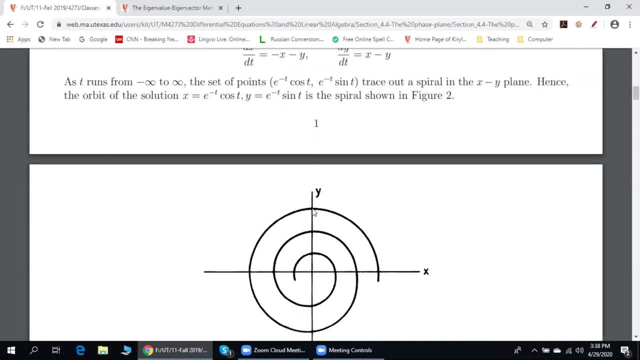 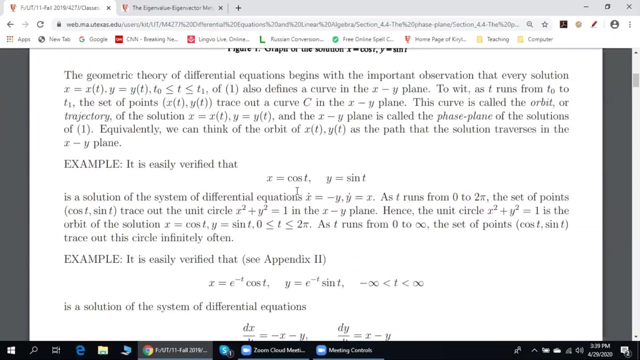 this, Agree, Yeah, Keep going. One can see that if you plug in, t is equal to pi, we will be here, and then this distance will be even smaller than this distance, and so on. Okay, cool. So in these two examples we trace the orbit using college algebra and trigonometry tools. 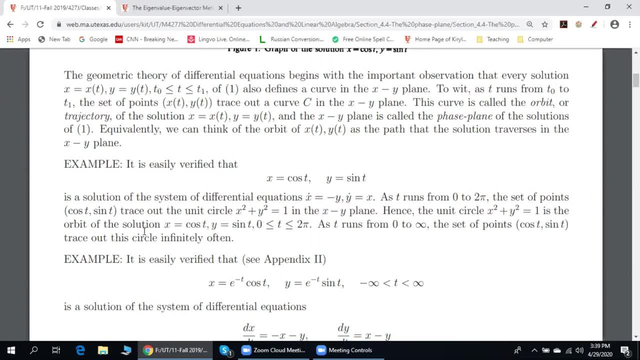 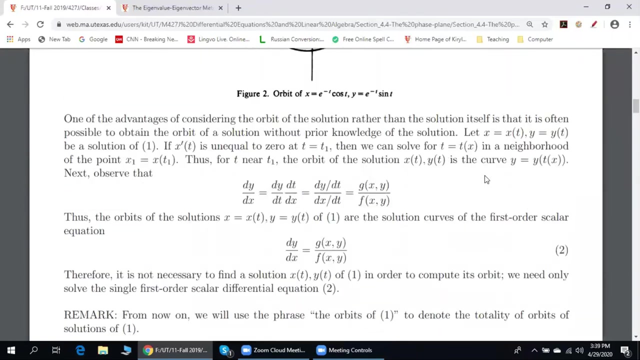 In example number one we managed to exclude t completely. In example number two we excluded parameter t partially. But anyways, in these two examples we applied only college algebra and trigonometry tools. In the second part of this handout we use a totally different method. So this handout 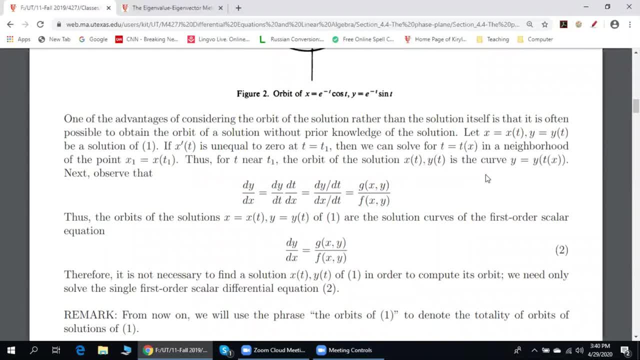 consists of two parts. One is the trigonometric method and the other is the trigonometric method. Part number one: we exclude t completely or partially, using college algebra or trigonometric tools. In part number two, we will use calculus. Let me go back to this. So we click on calculus. 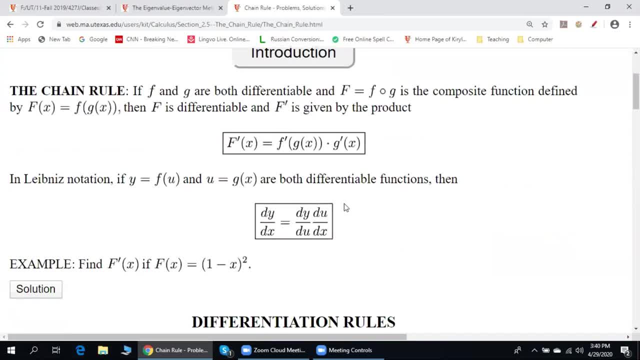 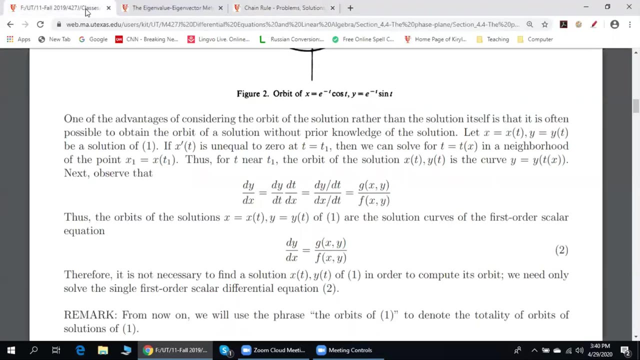 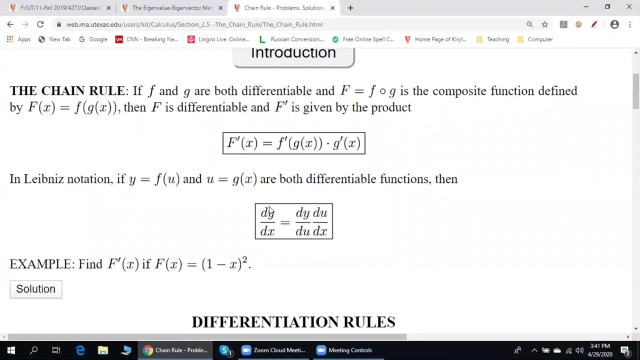 and chain rule. Please take a look at this formula: dy dx. This is dy du times du dx- This is chain rule. In our case, let us replace u by t. So if in this formula we replace u by t, the formula becomes dy dx, which is exactly over here, is equal to. 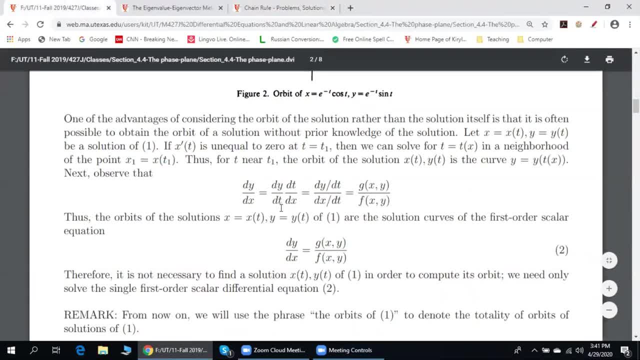 dy dx. So if in this formula we replace u by t, the formula becomes dy dx, which is exactly over here, is equal to dy dx. Now let us think about dT dx as about the normal algebraic fraction, As we discussed. 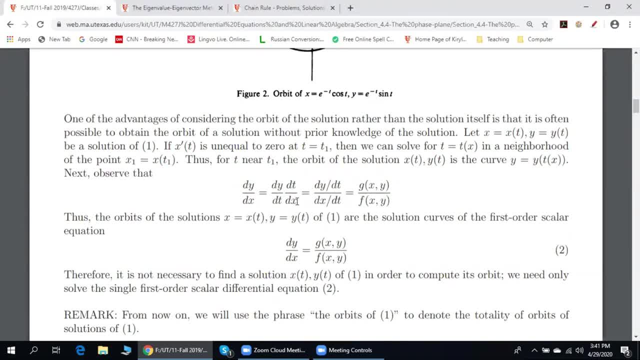 we can do it if we think about dT and dx as about differentials. Now let us use college algebra. When we multiply by dt divided by dx, it's same as we divide by dx divided by dt. Lastly, observe that dy- dt is g of xy. 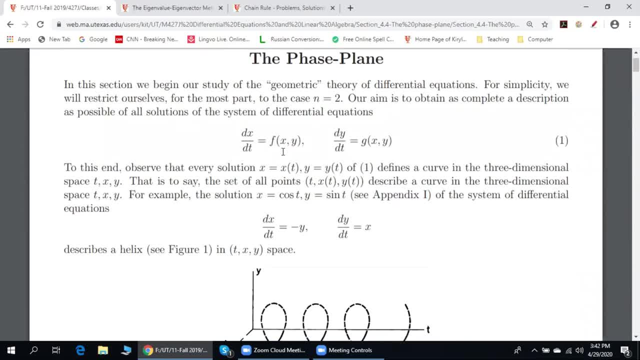 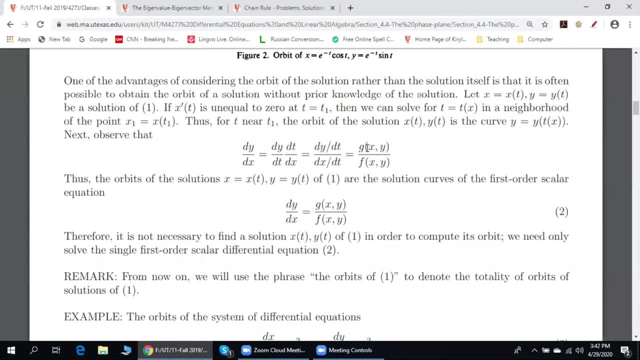 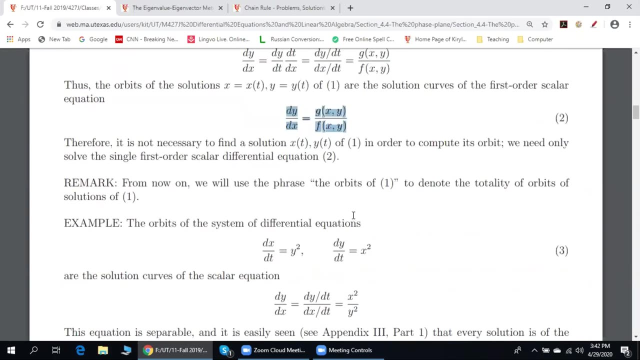 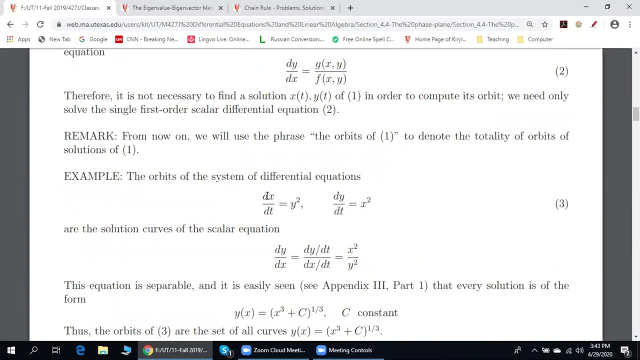 dx. dt is f of xy. Okay, Conclusion: dy: dx is g divided by x. It's exactly what is written here. Here's an example. Let us consider this system of differential equations. Note that we do not know how to solve this system. 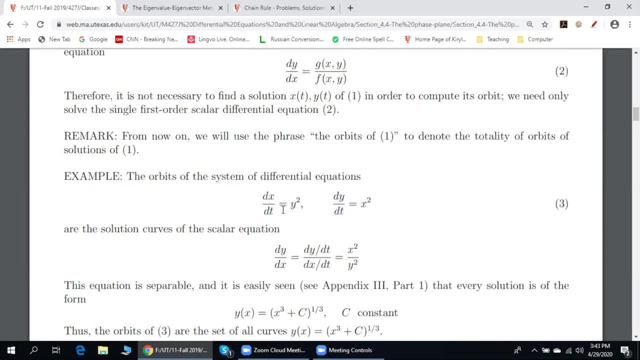 because this system is nonlinear. We have x square, we have y square, but we don't really need to solve it in order to find orbits. Instead, let us use these formula: dy dx, which is on the left-hand side, is dy dt, or which is x square, done? 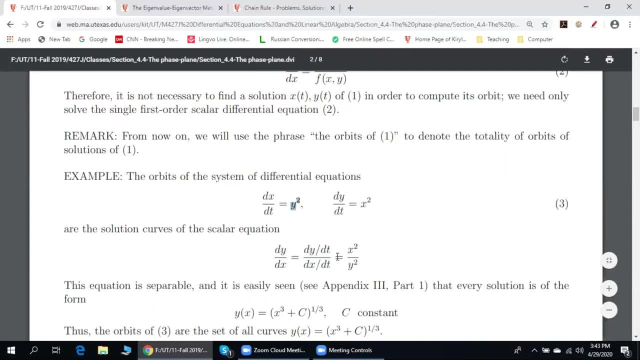 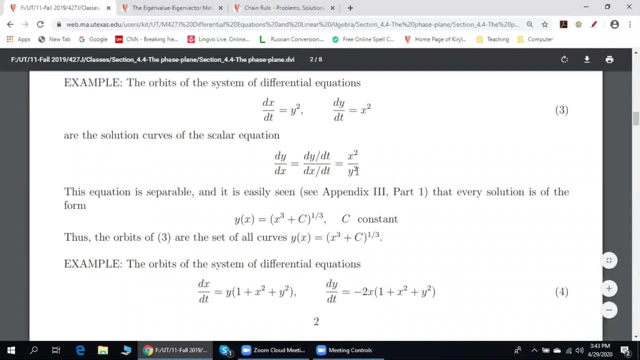 divided by dx, dt, which is over here done. Lastly, observe that dy dx is equal to x square or y square is a separable differential equation. We show how to solve it in Appendix 3.. Here is the general solution of our equation. 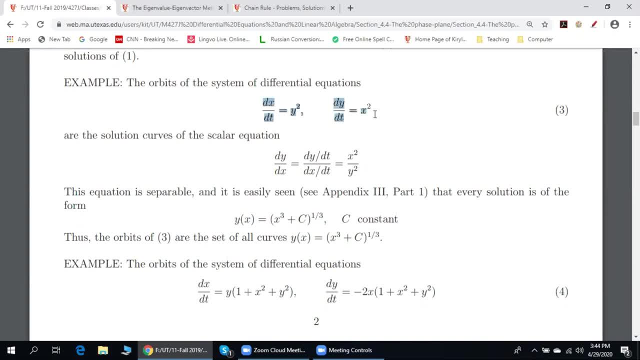 Therefore, the orbits of the system are the set of curves. Y is equal to cubic root of x, cubed plus c. And now, in order to sketch these orbits, you can use, for example, Wolfram alpha. Let us go to Wolfram alpha. 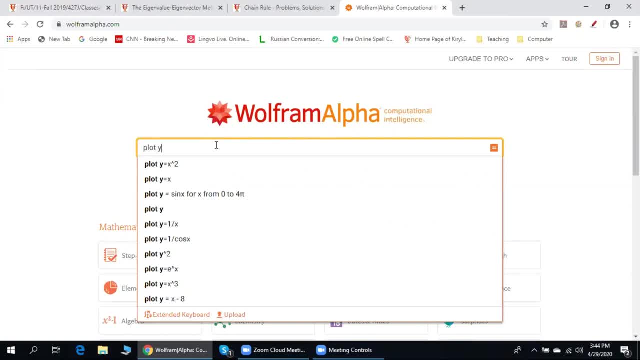 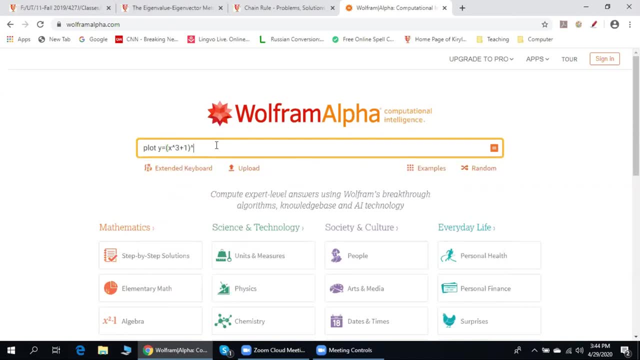 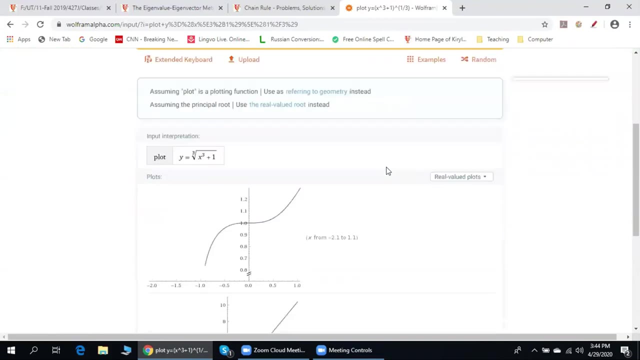 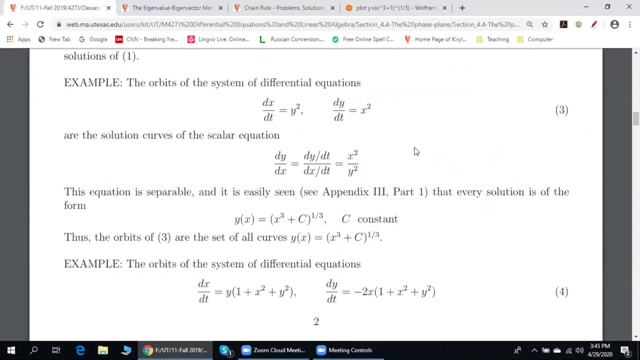 So we type in plot: Y is equal to x cubed plus one to the power 1- 3rd. And here is a particular order And we can write a particular order for the orbit. Any questions here? Wait, can you reiterate what the significance of an orbit is? 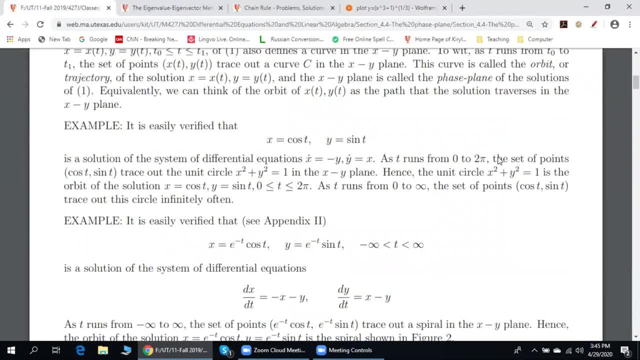 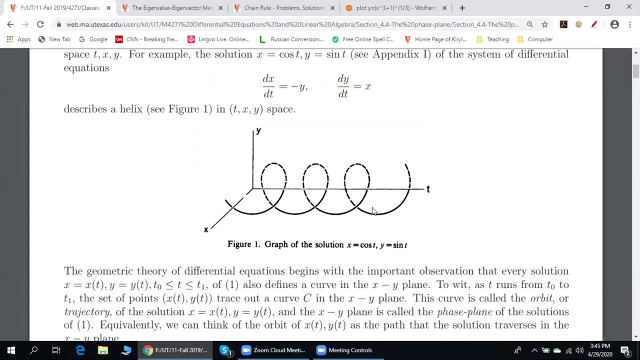 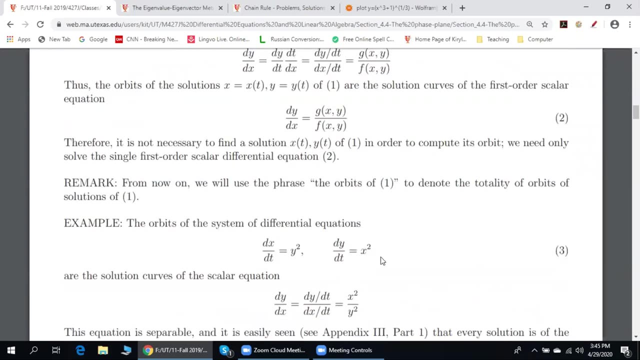 An orbit allows us to visualize solutions. An orbit is a projection of a three-dimensional curve on the x-y plane. So if we consider a particular solution of this system, it is given as x cubed plus t, y cubed plus t. 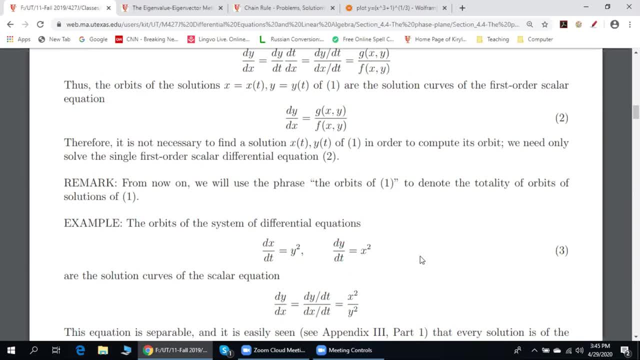 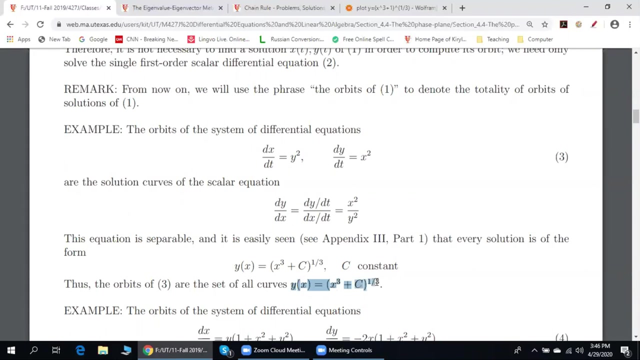 and if we consider the following triples: t, x cubed plus t, y cubed plus t, these points will trace a three-dimensional curve. If we project these three-dimensional curves on the x-y plane, the resulting two dimensional curves are graphs of these equations. 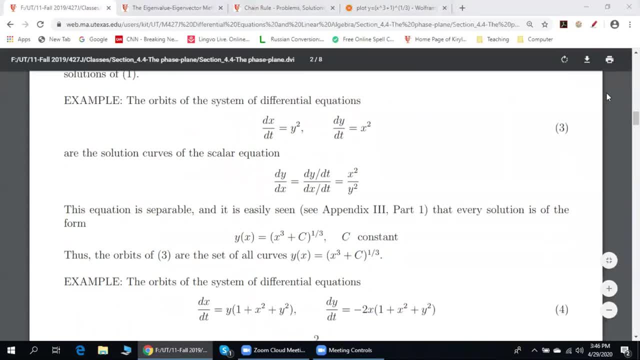 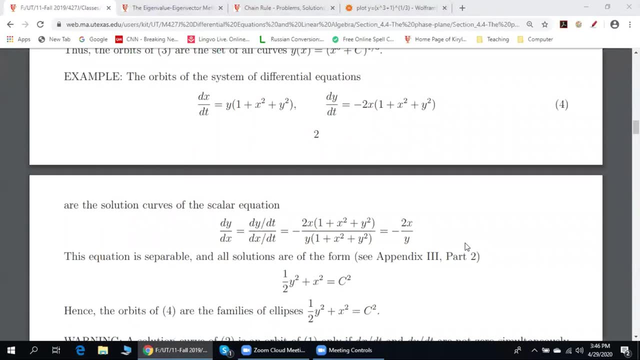 Was that your question? It was yeah, Thank you. Here's another example. We have a system of differential equations. We apply the same idea: dy dx is equal to dy dt, which is this, over dx dt, which is this: 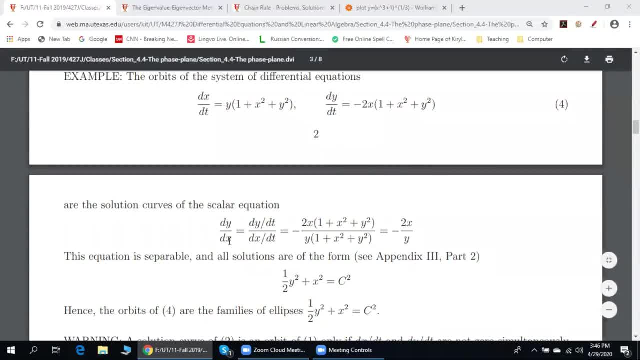 We cancel out the common term and the resulting equation is a separable equation. We solve it in Appendix 3, Part 2.. The general solution is: 1 half y squared plus x squared is equal to c squared. So the orbits of our system are the families of ellipses. 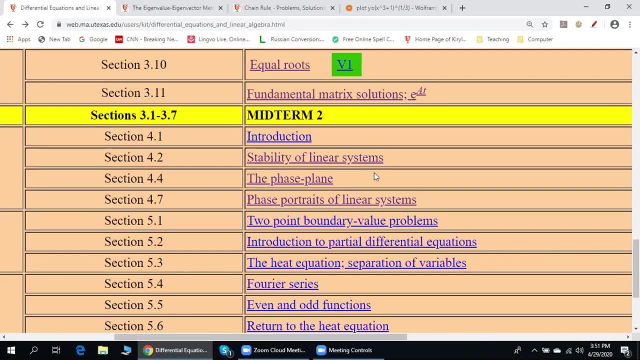 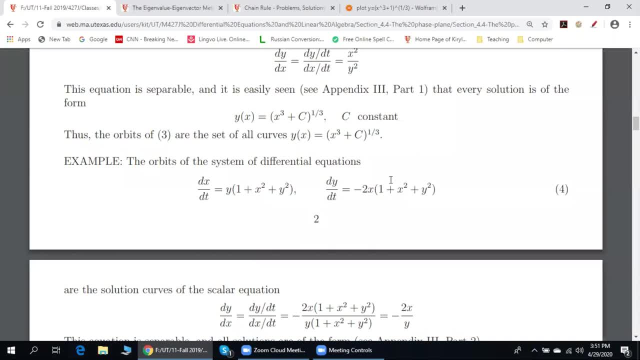 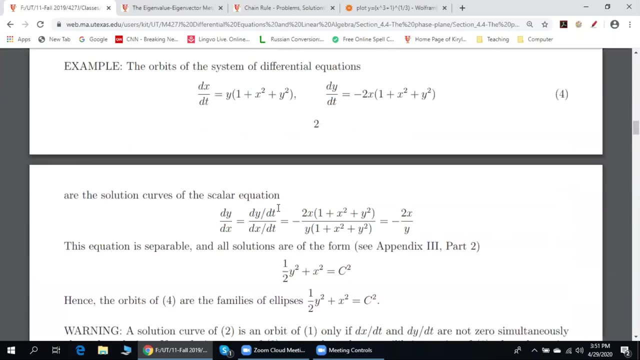 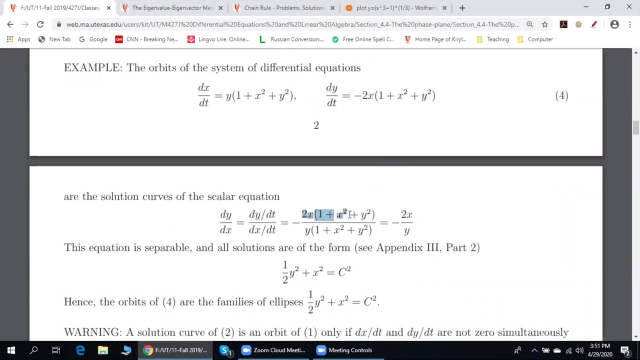 Any questions? Professor, would you mind redoing the last example we did. Are you talking about this example? Yes, So we apply. We apply this formula. By this formula, dy dx is equal to this, which is over here, divided by this, which is over here. 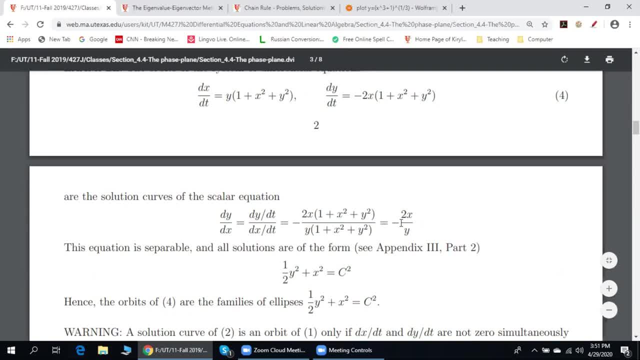 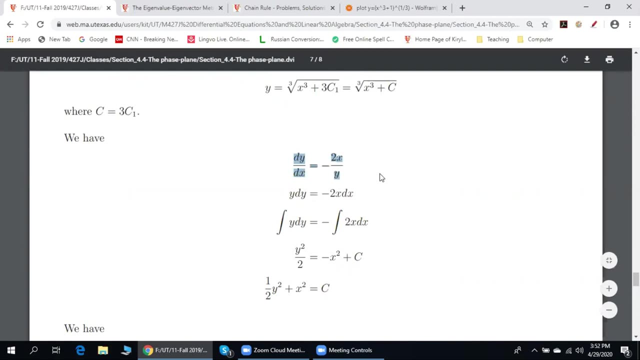 We cancel out the common term and the result is negative: 2x over y. Now, what we see in front of us here is a separable equation. Please take a look. We look at Appendix 3.. In order to solve it, here is this equation. 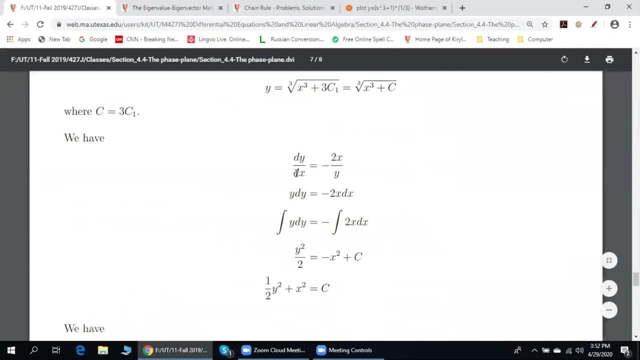 We move y to the left, dx to the right, Done, We integrate both sides. Anti-derivative of y is y squared over 2.. Anti-derivative of 2x is x squared. And lastly, if we move negative x squared to the right, 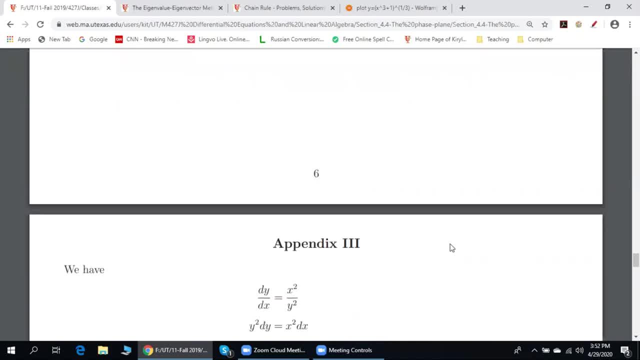 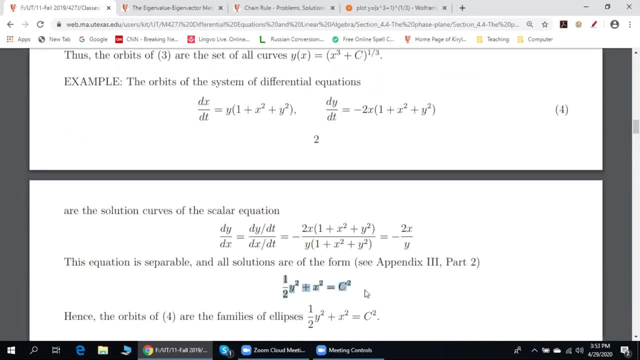 we solve this equation, We get exactly what is written over here. This one. The graphs of these equations are ellipses. Did I answer your question? Yeah, Also, why is c squared? Let me start with an equation of a circle. 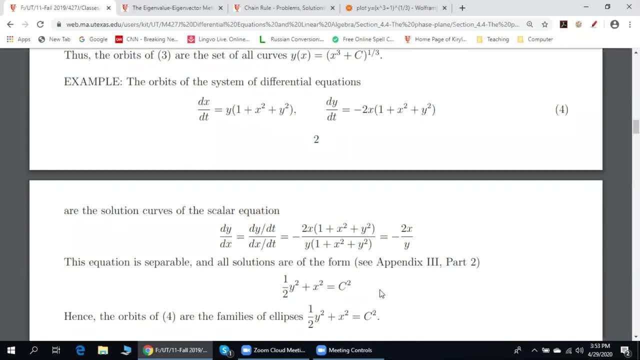 The standard way to write down an equation of a circle is: x squared plus y squared is equal to r squared. So basically we follow the same pattern here and we put here c squared. Okay, sure that makes sense.